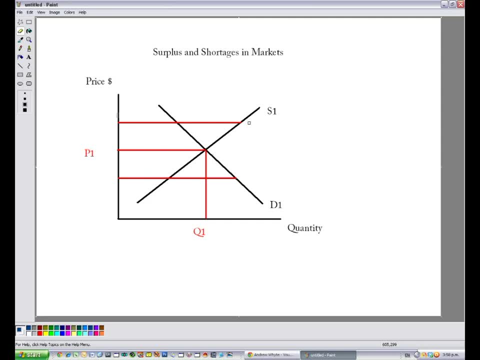 as the price increases, a supplier is willing to supply more, hence the upward sloping line and a greater quantity of goods and services produced in this particular market. But what would happen if we decided to set that price Outside of this market equilibrium which is right here where they join? This is the natural. 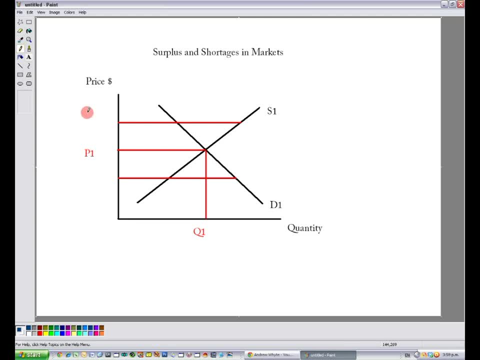 price level of this market. If we decide that we're going to go P2 up here and set the price, you may decide this is what you need to charge to make a living. It may be a market where the government is setting the price. It could be other reasons that you set that particular price. 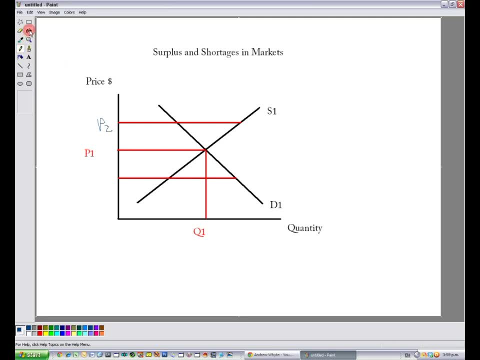 What you will get in this graph is the price that you're going to set. This is the price that you're going to get in this particular area. here is what you call a surplus, meaning that there's a stalemate existing between the consumers and the suppliers. You end up with a surplus of goods and services. 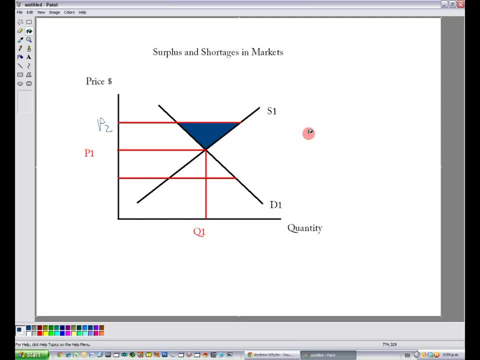 Now you've seen this- in warehouses stocked full of product they simply can't sell because the product is too expensive. Eventually, what will happen is the suppliers will move their prices down to match what the consumers are demanding. The market will once again be in equilibrium. but what happens if you price your goods and 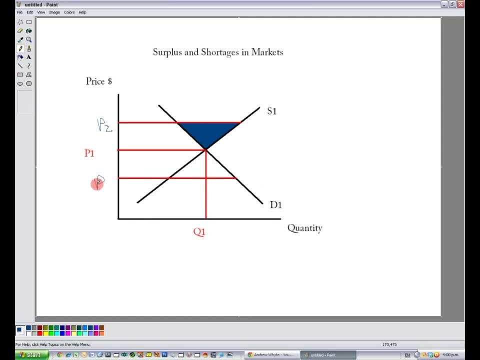 services too low. This could happen for various reasons too. The consumers are willing to pay a lot more than the supplier actually wants for their goods and services Interesting, but what is happening here is that you have got a shortage in the market. This market will. 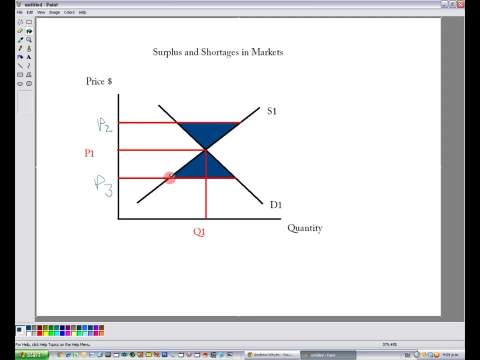 eventually correct itself. as a supplier realizes that the consumers are willing to pay a lot more, He will increase his price. He will increase his price. He will increase his price. He will increase his prices to match the actual market equilibrium here at P1 in huge numbers. 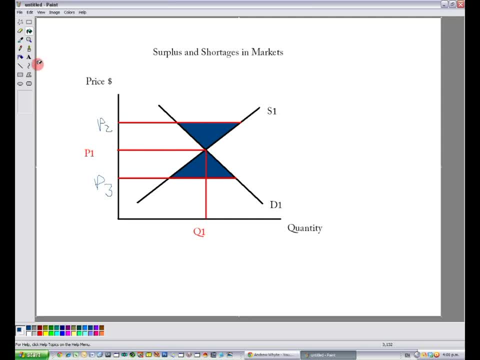 So, regardless of where these prices are set, in a free-market economy, there will be surpluses and shortages. that will quickly correct itself. in a market where prices are set either by the government or by the supplier, You will get a stalemate.